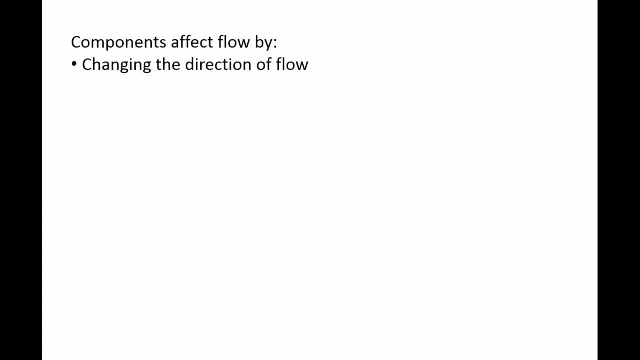 than HL major. In general, components affect the flow by changing the direction of flow, obstructing the flow and changing flow speed through varying the cross-sectional area of the pipe system. Pipe systems may have many components. Bends, elbows and tees are devices that change. 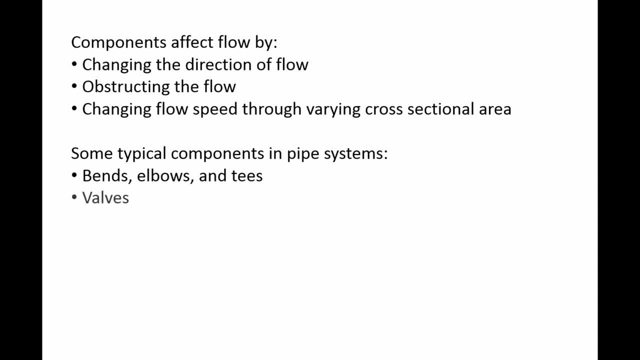 the flow speed of the pipe system. Pipe systems may have many components. Bends, elbows and tees are devices that change the flow direction. Valves are used to adjust flow rates. Expansions and contractions are used to slow down or speed up the flow and may occur suddenly or gradually. Entrances into pipe. 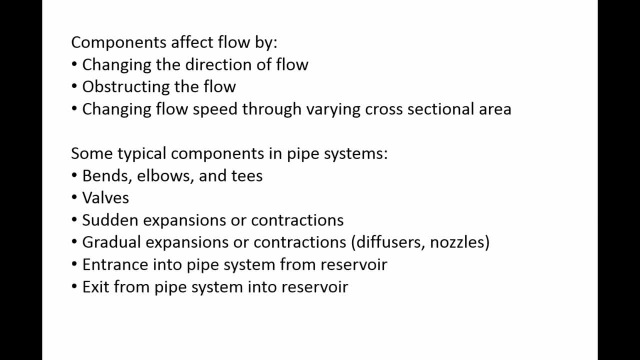 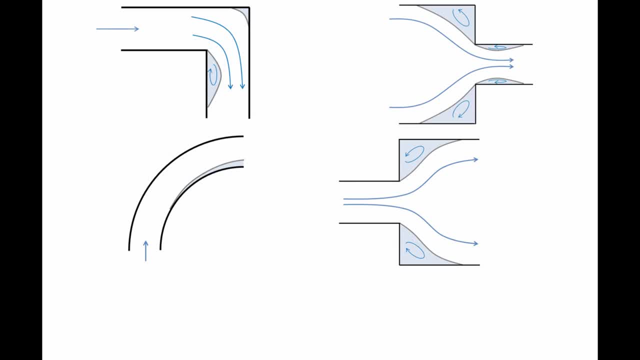 systems from reservoirs and exits from pipe systems into reservoirs are also considered to be components. Many components, such as the elbow bend, sudden contraction and sudden expansion shown here, cause the flow to change direction. This can lead to regions of separated flow, shown in blue, where eddies are formed. 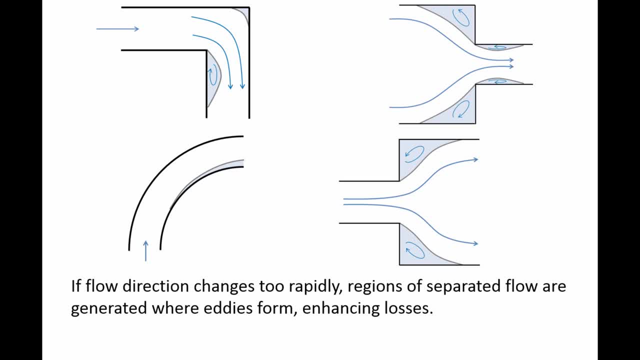 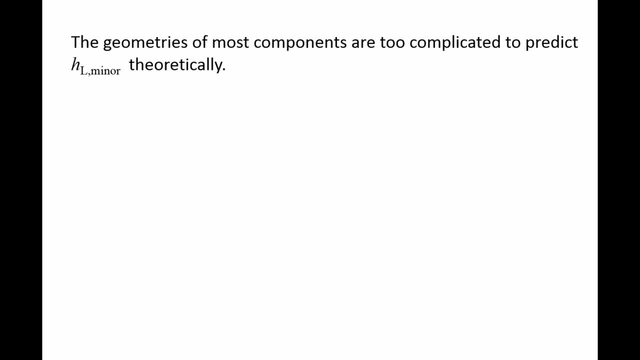 The presence of separated flow regions can greatly enhance losses in components. The geometry of many components are too complex to derive a theoretical expression for HL minor. Instead, the minor losses are calculated using an expression that is similar to the Darcy-Weisbach equation. For each component, the minor loss is equal to k times v average. 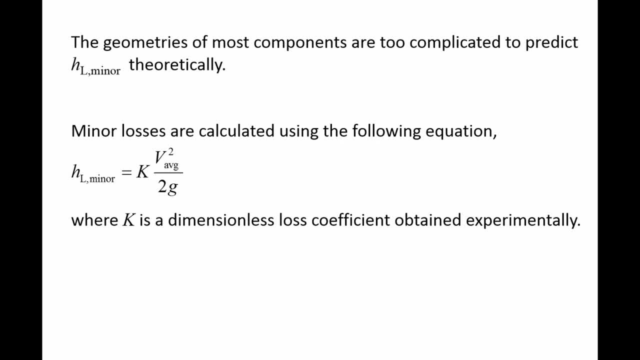 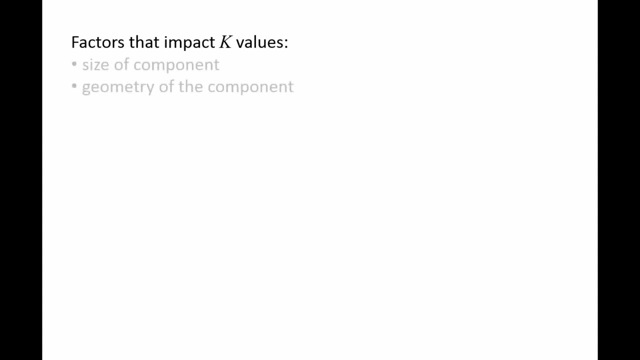 squared over 2g. k is the dimensionless loss coefficient that is obtained experimentally. Higher k values indicate higher losses for the same flow speed. There are many factors that can impact the loss coefficient: The size and geometry of the component, the Reynolds number, how the component is connected to a pipe. 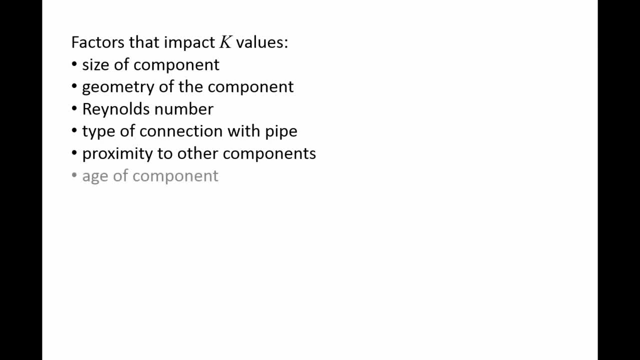 the proximity to other components and the age of the component can all affect the loss coefficient. k values are usually reported in tables, equations, charts or nomographs. For components that change cross-sectional area, the flow speed at the inlet and outlet will be: 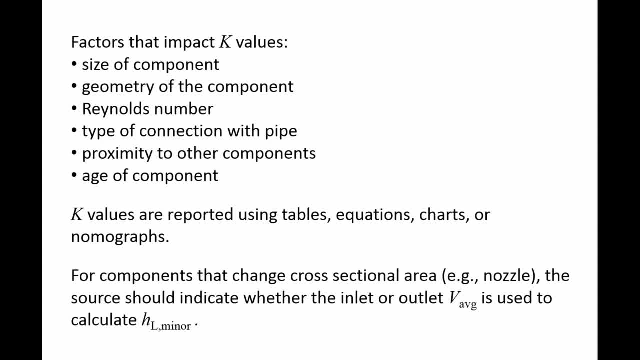 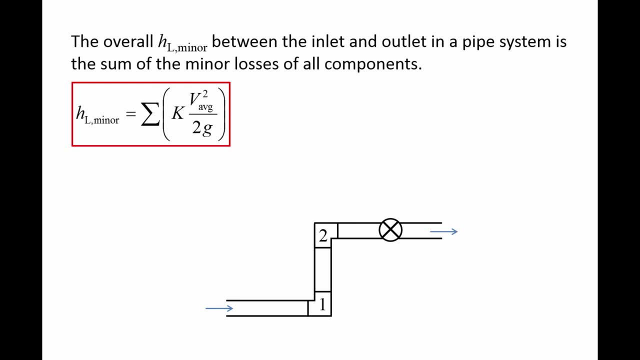 different For these components. the source that provides the k value should indicate whether you should use the inlet or outlet flow speed in calculating HL minor. Most pipe systems will have multiple components. When calculating the total minor losses for a pipe system, you need to add the contributions from all the individual components.